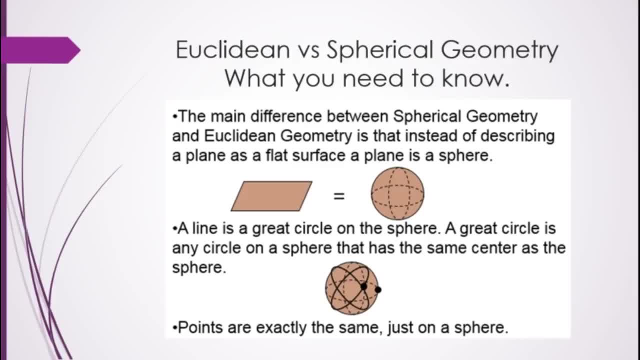 which is a sphere. So what do you need to know? As I go through these slides, fill in the blanks on your handout. The main difference between between spherical and Euclidean geometry is that in Euclidean geometry we said a plane is a flat surface. 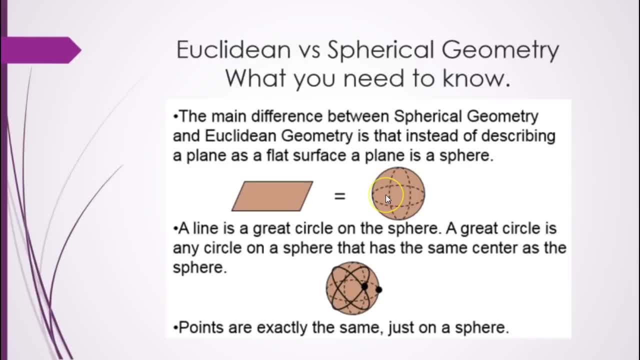 In spherical, a plane is a sphere. It's like the surface of the Earth. A line in spherical geometry is no longer just a straight line, It's actually a great circle. And a great circle is any circle on a sphere that has the same center as the sphere. 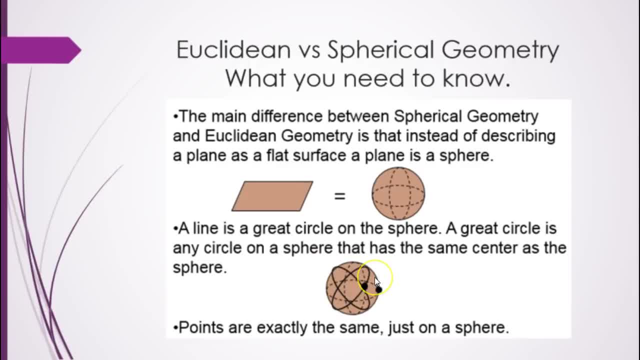 So each one of these circles drawn on here, So each one of these circles drawn on here, So each one of these circles drawn on here, is a great circle And we consider those lines And then points are exactly the same in both kinds. 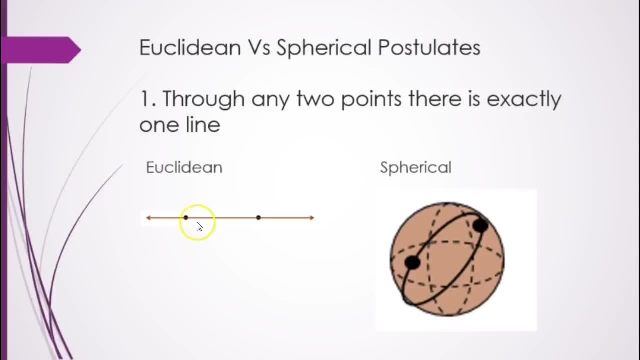 So things that are the same, Number one- through any two points there is exactly one line. One line or one great circle, because we said great circles are the same as lines. Through any three points there is exactly one plane. 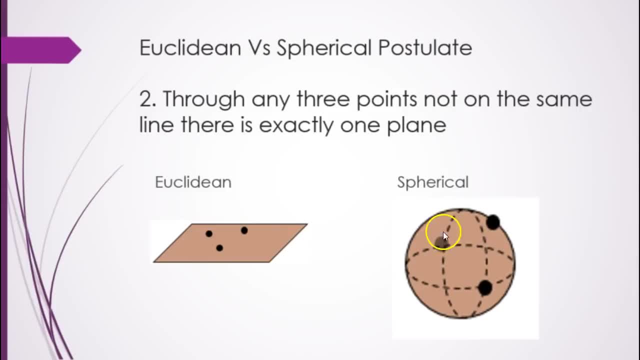 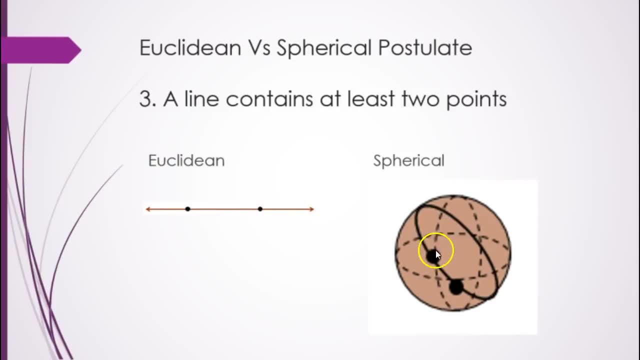 Here one plane, three points here makes one plane. One plane, one sphere. A line contains at least two points. Two points here, two points here. Remember a line is a great circle, Remember a line is a great circle. 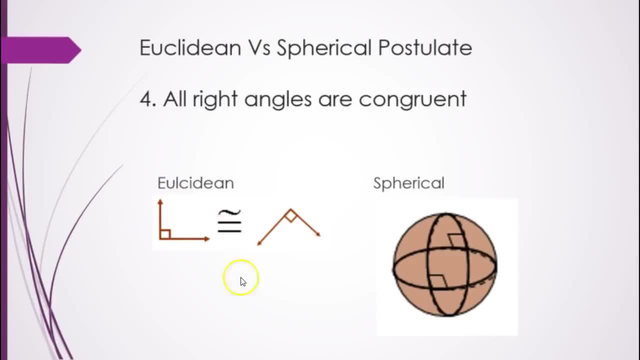 All right angles are congruent. We're used to right angles looking like this, but we can see here, right here, this is a right angle. it's 90 degrees and it's congruent to this one over here. it's 90 degrees and it's congruent to this one over here. 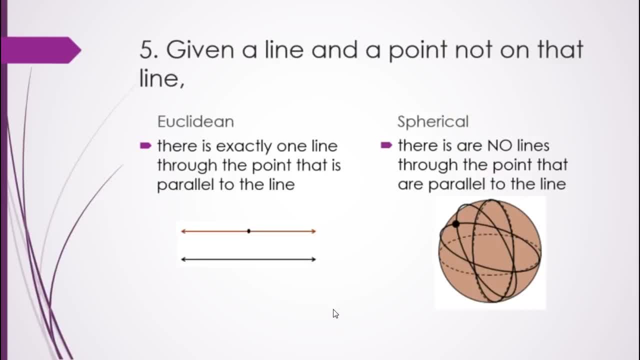 Now we're going to talk about ways that they're not the same. Now we're going to talk about ways that they're not the same. The first one is the right angle. The next one has to do with parallel lines. If we have a Euclidean geometry, 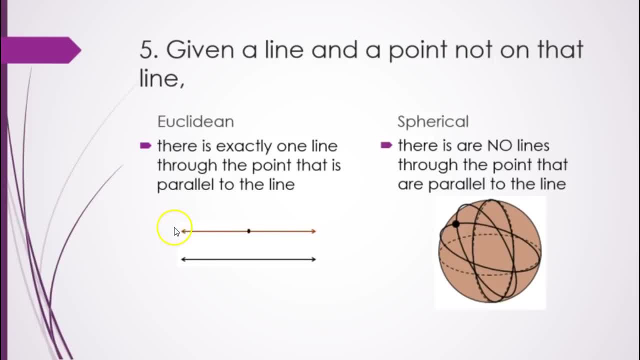 a line and a point that's not on the line. There's just one parallel line that goes through that point. However, if I try to do the same thing here, here's a line, it's this great circle and this point over here I could draw a couple of different great lines. 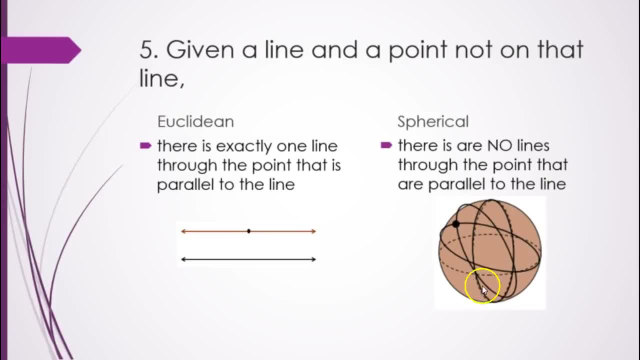 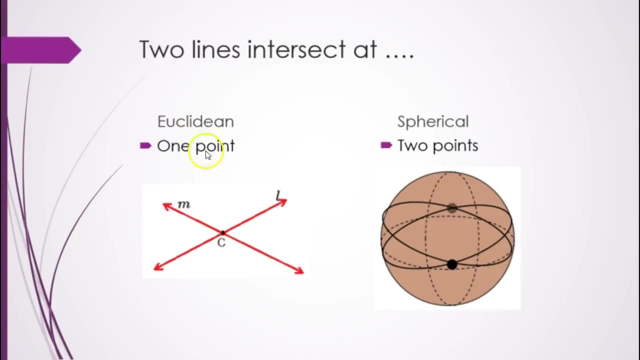 through this point, but none of them are going to be parallel to this line here are going to be parallel to this line here they're always going to intersect. so here there's one line that goes through it. here there are no lines that are parallel to the first one in Euclidean.